moistened soil. so it's free draining and great for my roots. I don't need to rake them up As I walk on them, they'll just break down and go back into the soil. But if your cores look like they're clay or they're a bit lumpy, got builder's rubble in them, something like. 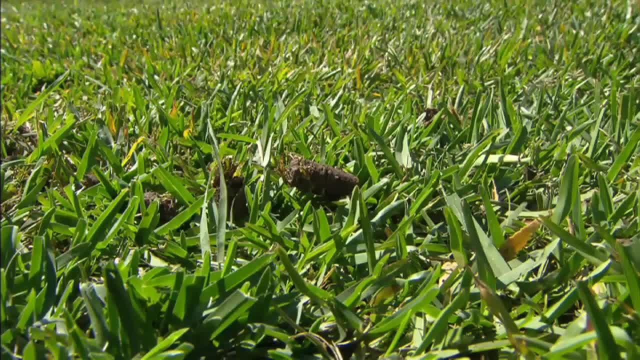 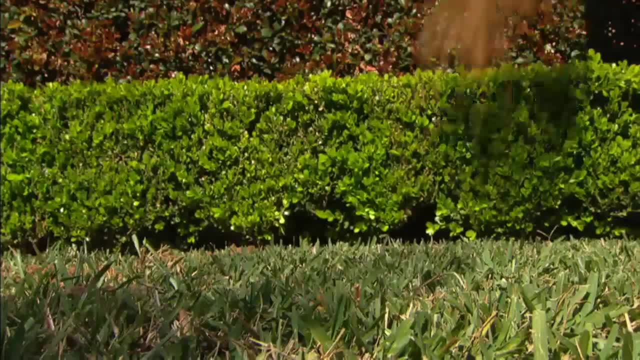 that you're better off raking them up and getting rid of them. You might think it's a good lawn, but it can be better. That's why I'm going to top dress. Just take out a few of the lulls and give the grass a little bit more of that free draining soil. And what? 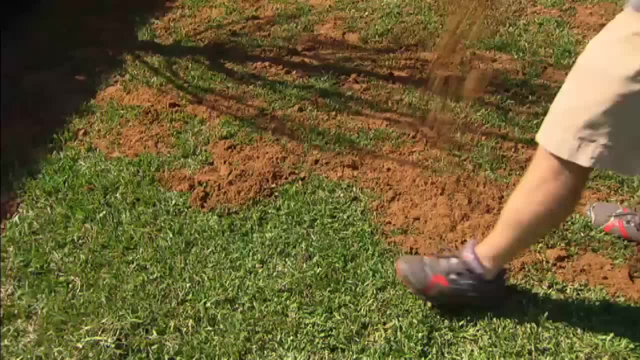 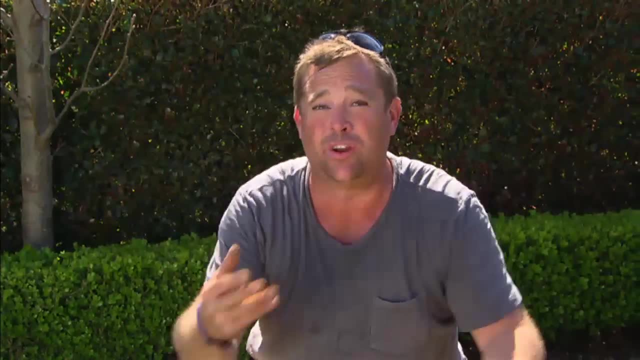 do I use? Well, you can call this ADP. It's 80% sand and 20% silt. It's exactly what gets flushed up onto the flats when a river floods, and that's why you see a lot of turf farms on the side of rivers. It's. 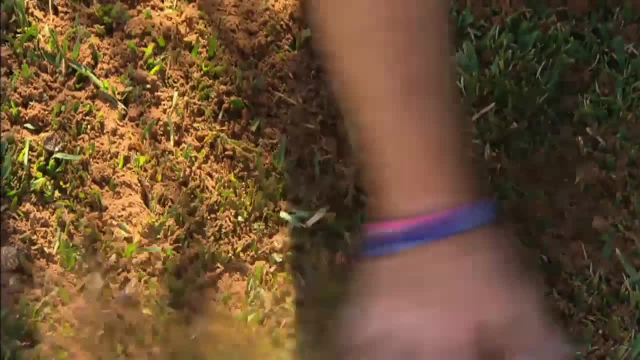 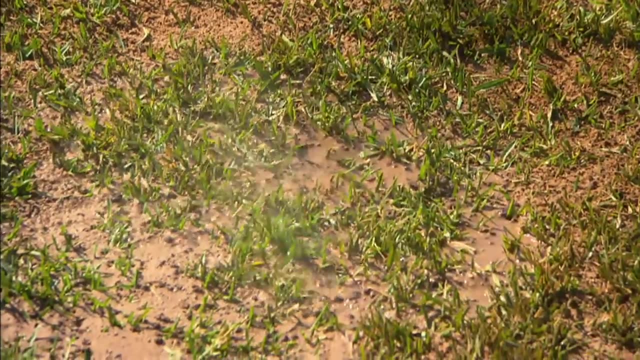 perfect for growing turf and it's nice and light, so established grass can grow through it. You want to water this every day until you can't see the soil anymore. If it dries out, it'll form a crust and the grass blades can't grow through it. On my back lawn I've 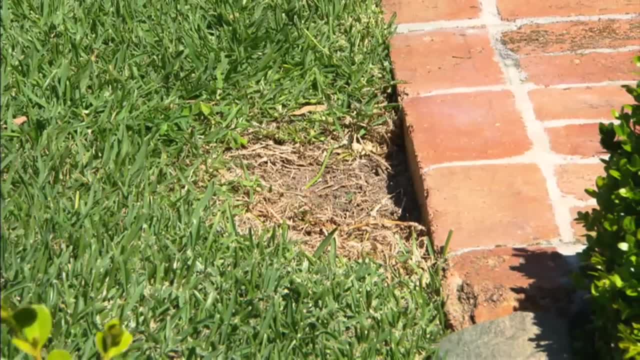 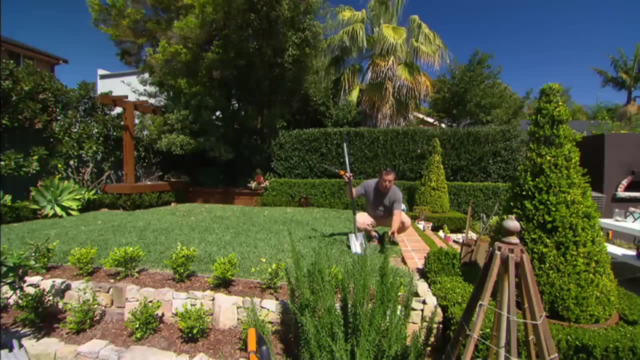 got some problems, but they're my fault. Just here you can see this semi-circle. Well, I had a large pot sitting on the brickwork and over the last 12 months it's killed the grass off and it's a really good example of a weak lawn or introduced weeds. You can see here. 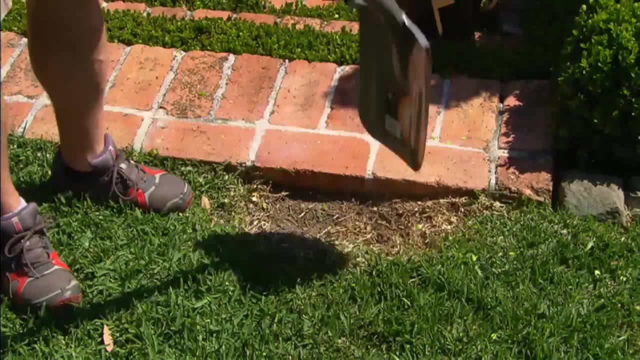 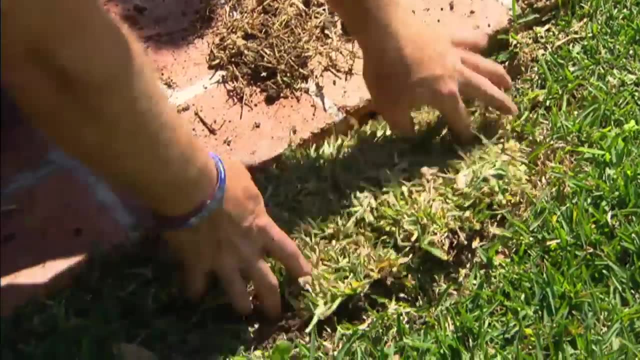 I've got a bit of onion weed and a bit of clover. I don't have it anywhere else in the lawn, so it's an easy fix. You can buy one roll of turf for around the $10 mark, cut it into any shape you like and repair it. Now, when it comes to fertilising, you've got 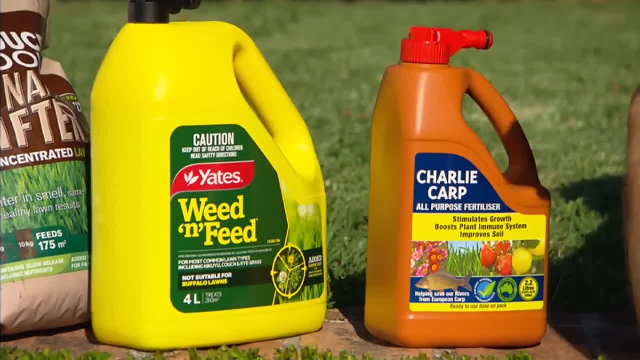 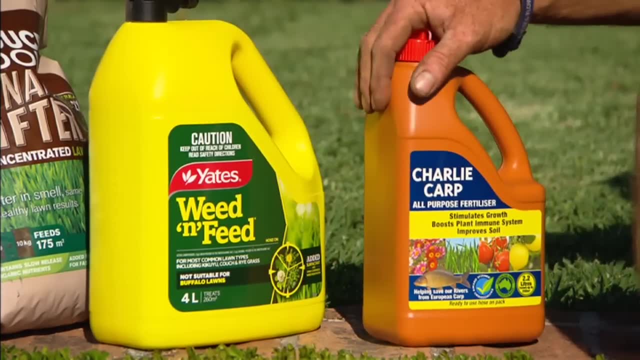 lots of choices. these days You've got liquid fertilisers that weed and feed. If you've got a really bad lawn, well then I recommend using one of them. It'll knock the weeds out and help the grass grow, But what I like to use is a liquid fertiliser that can be drawn. 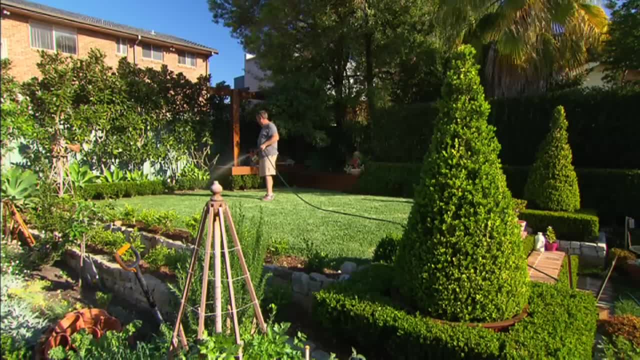 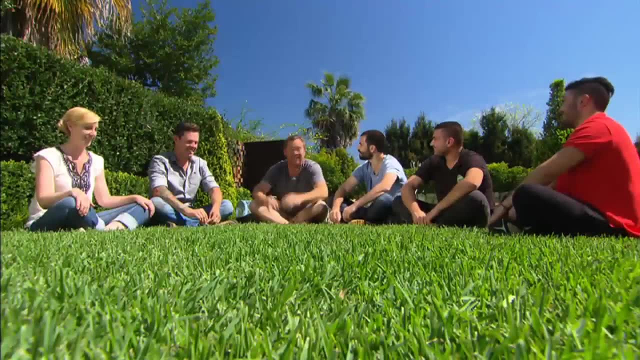 up between the foliage and the root system, It makes it look really good really quick. If you treat your lawn like it's a garden bed- after all it is a plant- you're going to have a fantastic lawn come Chrissie. Alright, congratulations, guys. Now repeat after me. 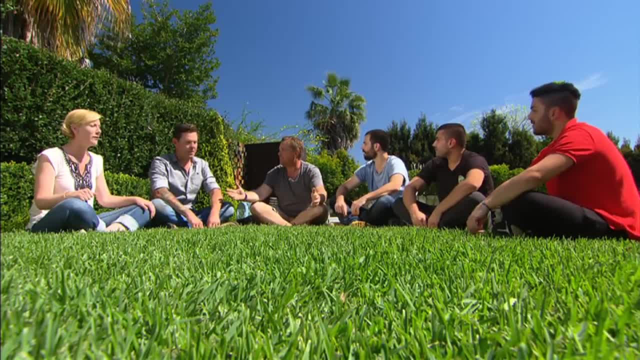 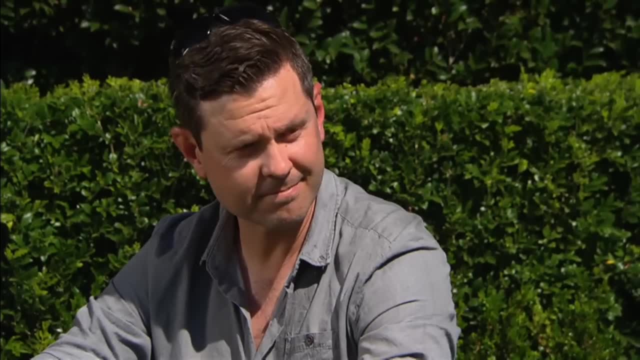 I deserve a beautiful lawn. I deserve a beautiful lawn. Round of applause for you guys. Alright, now next week's meeting is at the same time. It's how to deadhead your annuals, And no mate, we won't be using chainsaws. Go home. 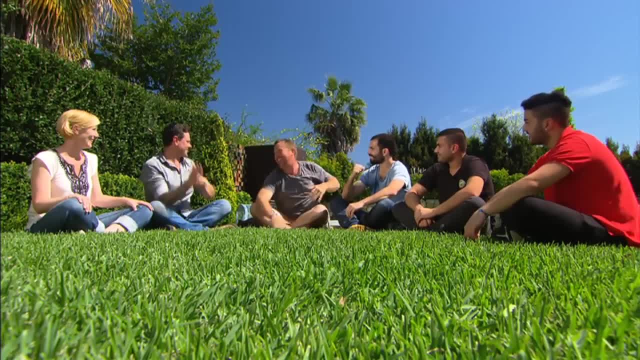 and love your lawn High five.